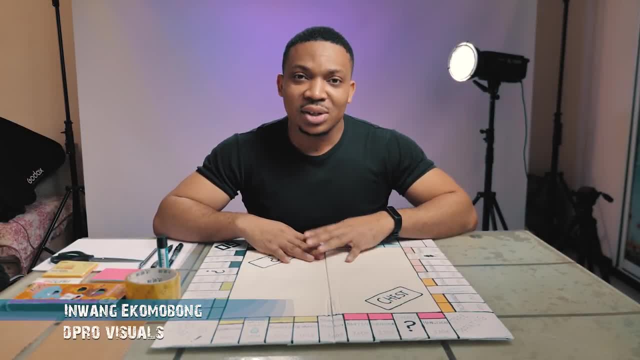 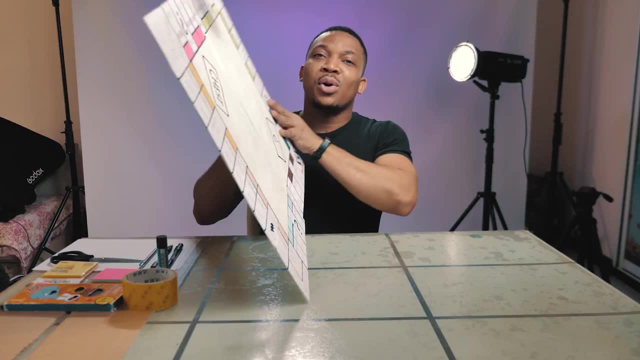 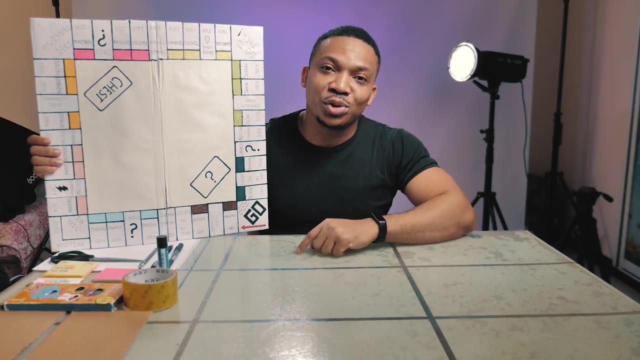 Hi guys, this is Nwanyi Okomobo, and welcome to Deep Road Visuals. So today I'm going to be showing you guys how to use simple materials you find around your house to make a simple monopoly board. As you can see, this is clean and neat, and I'm going to show you right now how to do it. 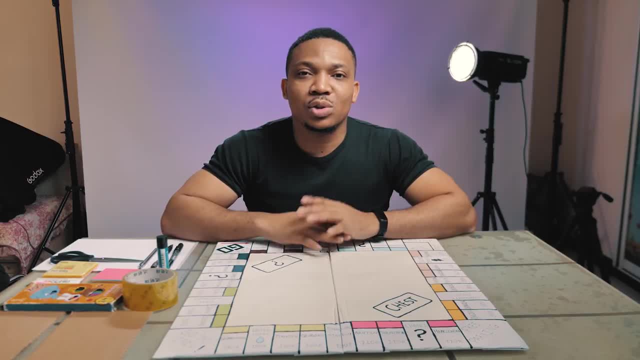 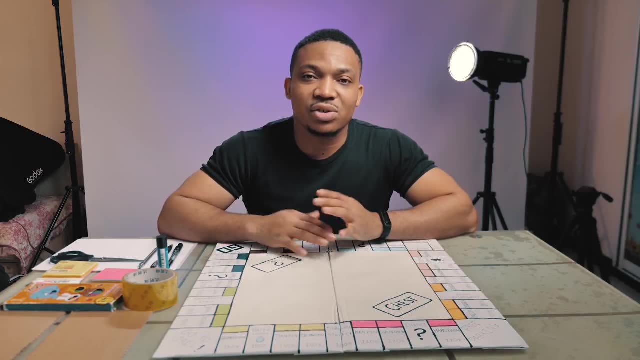 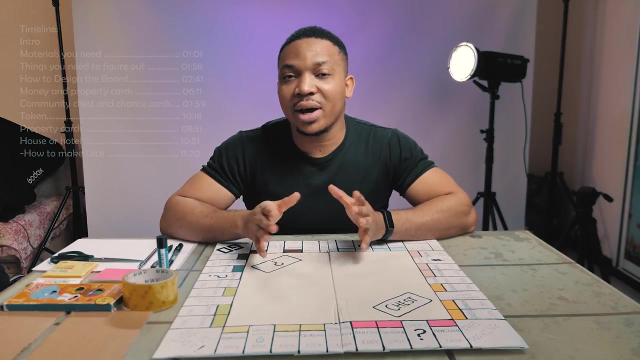 yourself In the midst of this pandemic. we need to have something to do to keep ourselves busy, and in my previous video I talked about why it is necessary for us to stay at home and certain things we could do to keep ourselves busy. So, as they say, all work and all play. 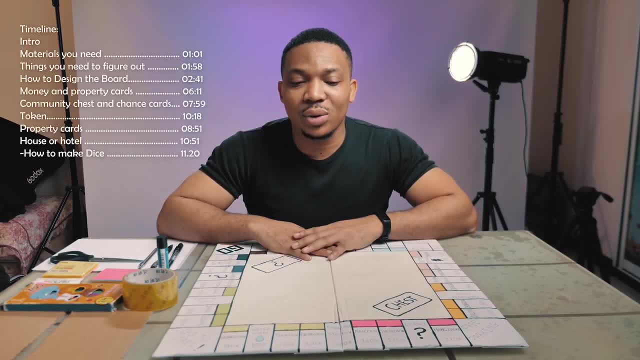 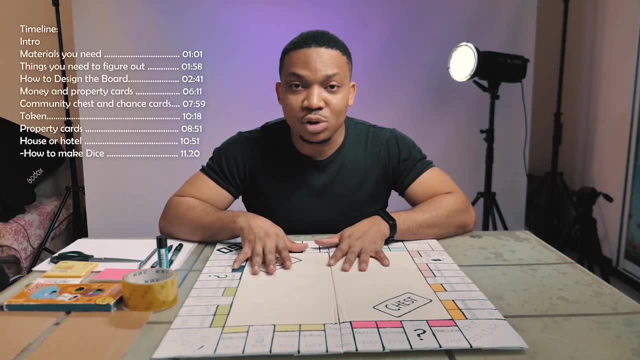 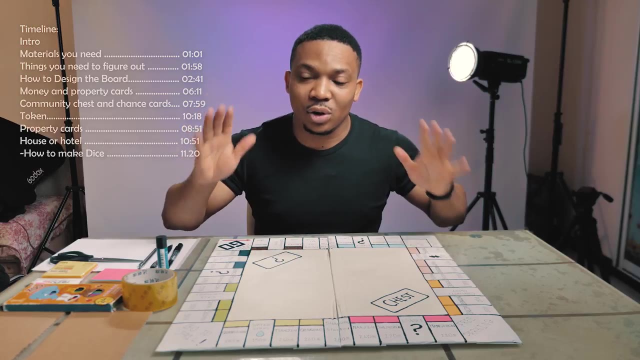 make Jack a dull boy. So today I want to show you guys how you can make a simple game which is fun to make with your friends, your families, the kids. They're going to love it so much. and this is a very simple game you could make using simple materials you find around your house. 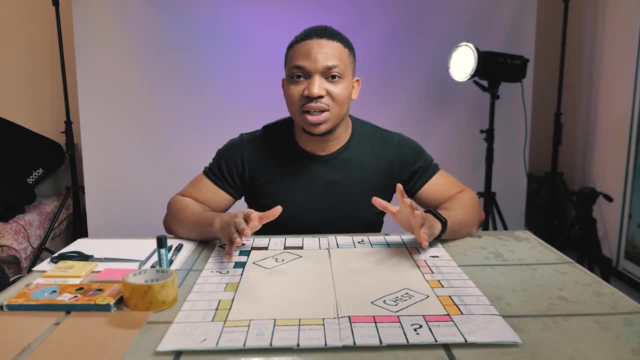 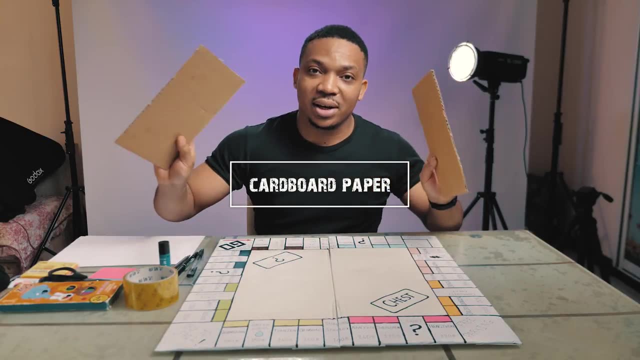 So let's get started. So we're going to start from five materials which you're going to need in making this monopoly board. You're going to need cardboard paper, which I have two of them here. Don't worry, I'm going to tell you why they are two. You're going 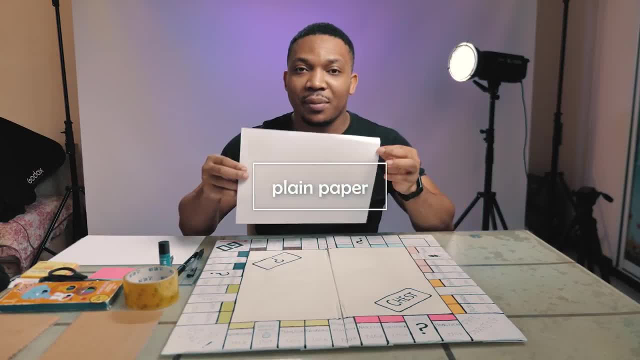 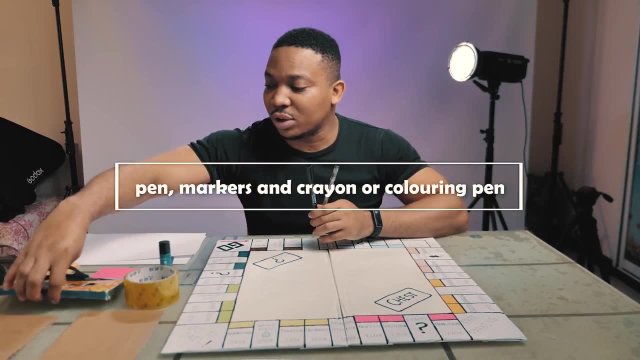 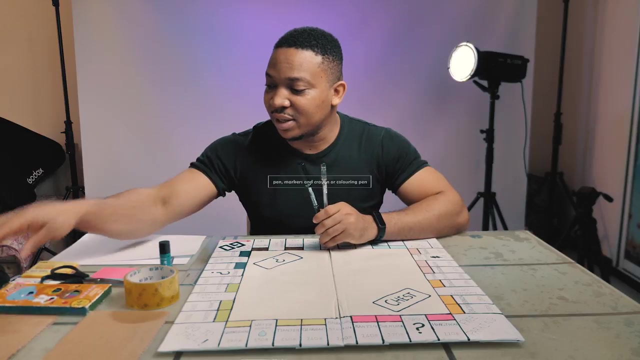 to need a plain sheet of paper. I'm using A4 for this. You're going to need paint markers and crayons or coloring paint If you have them in different colors. it's going to come in very, very handy. And I also use coloring papers- different colored papers, which I have here. 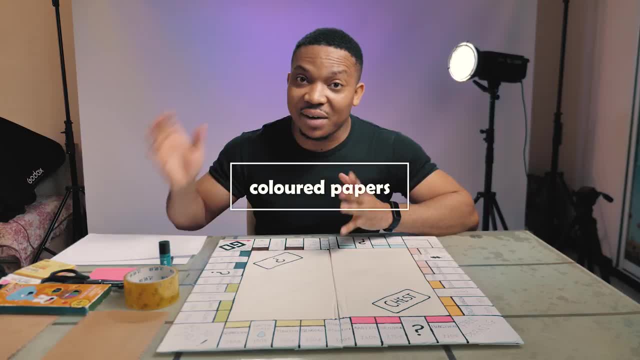 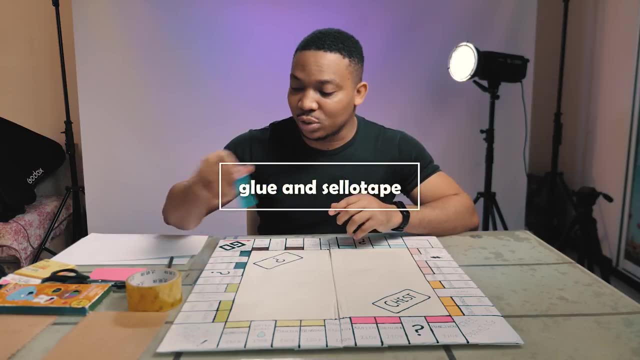 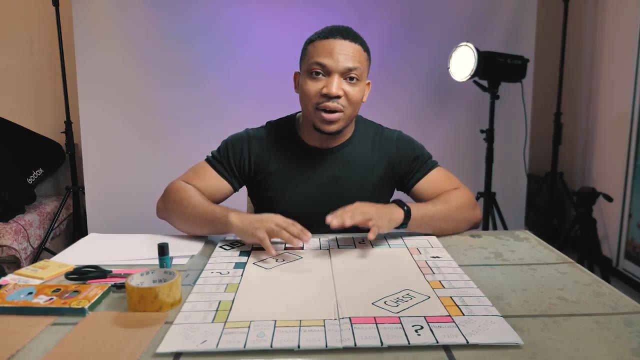 but it's not necessary if you don't have them, But if you have them, you can also use it too. So I also have glues here- This is for sticking things together- and also a pair of scissors. So basically, this is all what you need, and don't panic, don't be afraid If you don't. 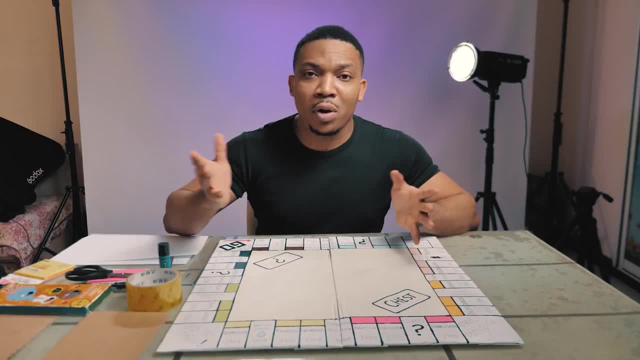 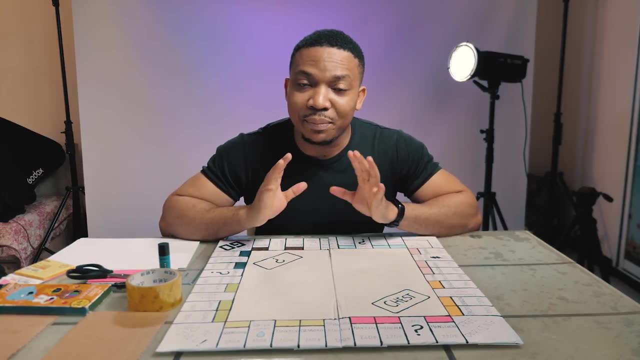 have any of these things. feel free to be creative and come up with things, things around you, to make the best out of your board. There are five things you also need to have at the back of your mind before embarking on this fun exercise. So the first thing is how to make or design your board. 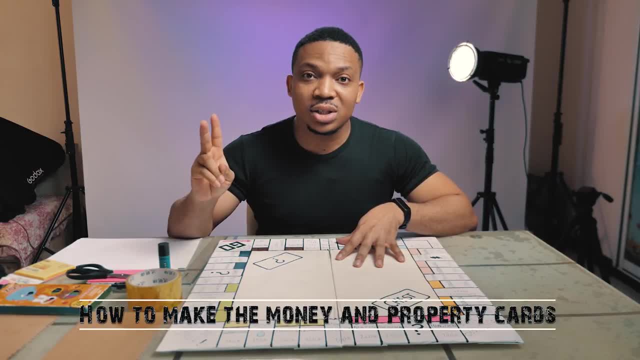 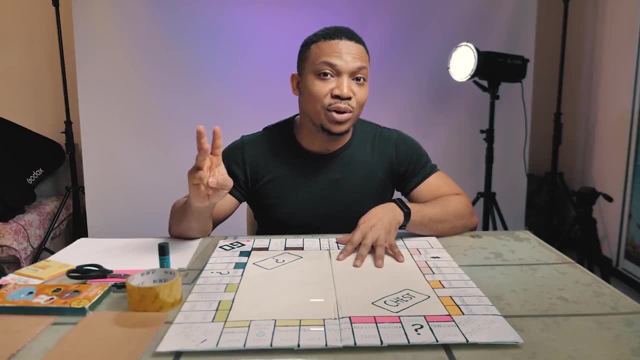 Secondly, you're going to need and figure out what you're going to use in making the money and also property cards. And third, you're going to also try to figure out how you're going to make your dice for rolling. And fourth, you're going to need to figure out what you're going to use for. your dice. And fourth, you're going to need to figure out what you're going to use for your dice for rolling. And fourth, you're going to need to figure out what you're going to use for your dice for rolling. And fourth, you're going to need to figure out what you're going to use for your. 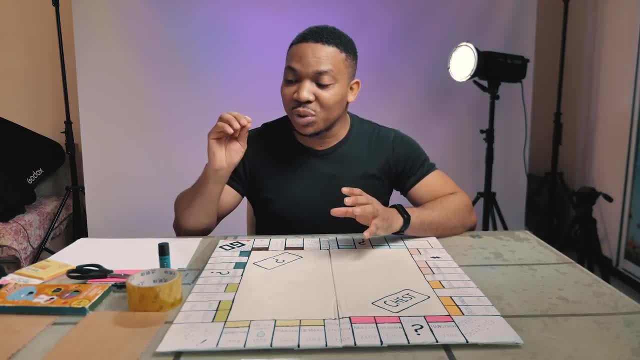 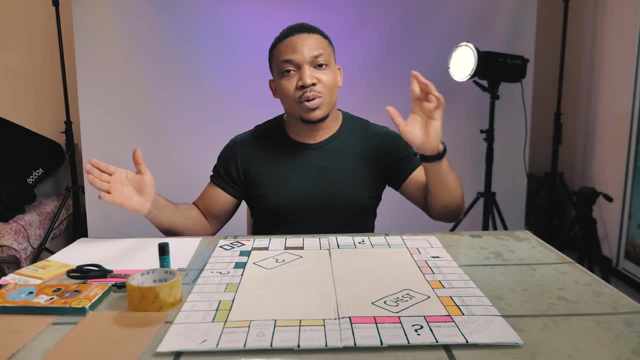 token And the last, what you're going to use or what you will need for houses or hotels. So if you figure this out, then we are done. So I'm going to walk you, step by step, what you need to do at each stage. So first of all, let's talk about the board. 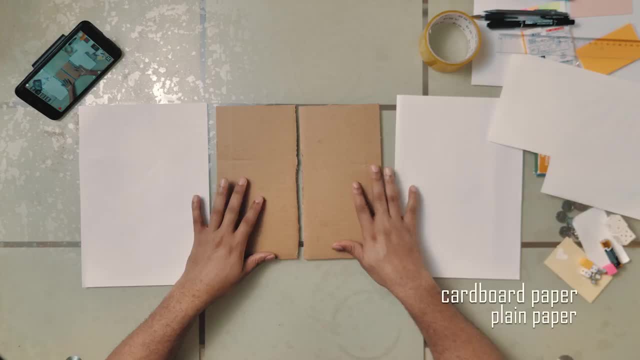 In making the board, you're going to need a cardboard paper and also plain paper. For the sake of this video, I've decided to resize mine and make this 25 cm by 25 cm. For the sake of this video, I've decided to resize mine and make this 25 cm by 25 cm. 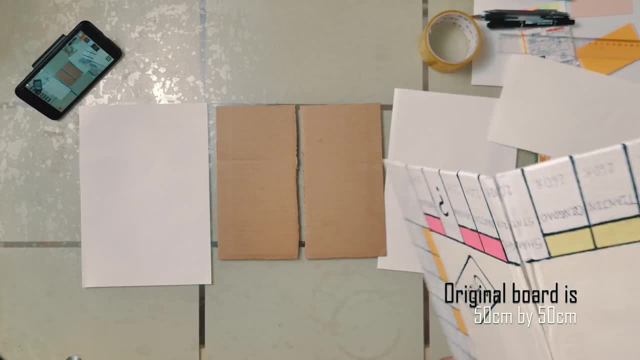 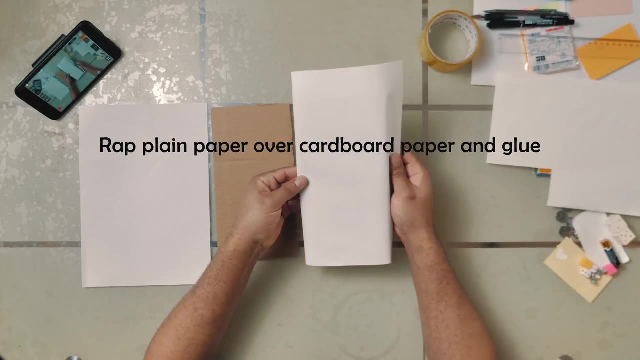 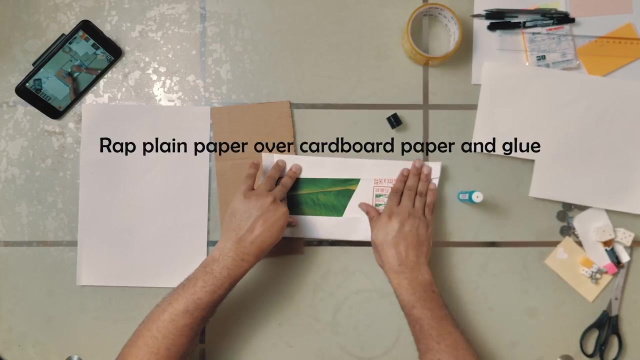 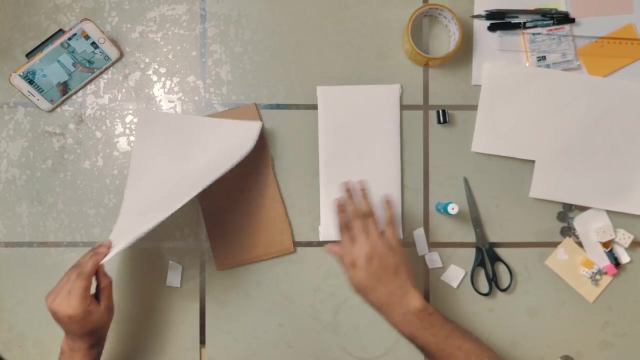 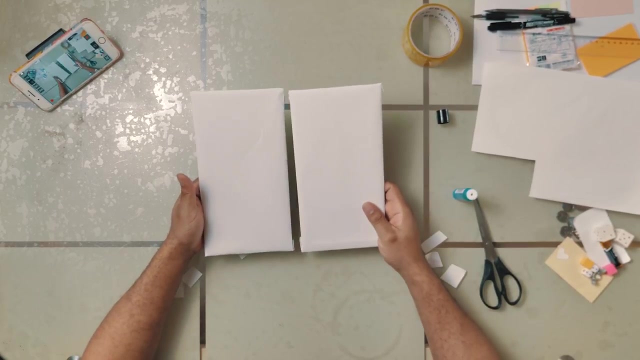 But the actual board is actually bigger than this. It's 50 cm by 50 cm, So you need a perfect square. So we're going to do the same thing for this other board as what we did here. So, yeah, you have two surfaces. Why I separated both of them is because 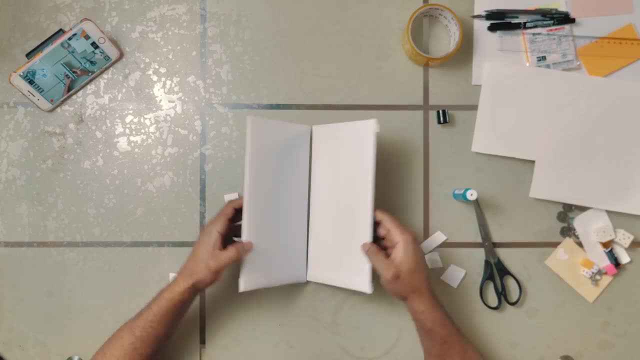 you might need to close the board, And if you get just a single plain cardboard paper, you're going to have an issue with the center. So, having achieved this, we're going to go in with a cello tape behind and stitch this together. 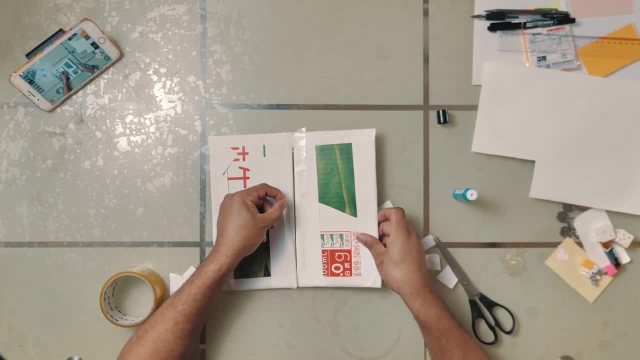 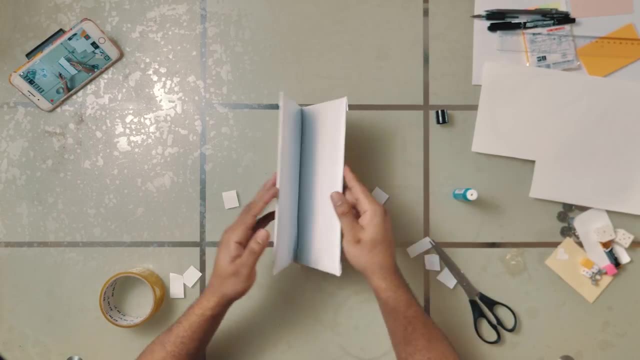 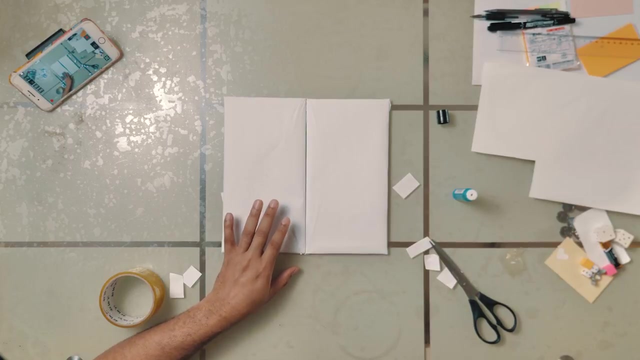 As you can see, we have a nice board which you can close and you can open. As you can see, we have a nice board which you can close and you can open. So the next thing we're going to do is to draw our different houses, or the different properties. 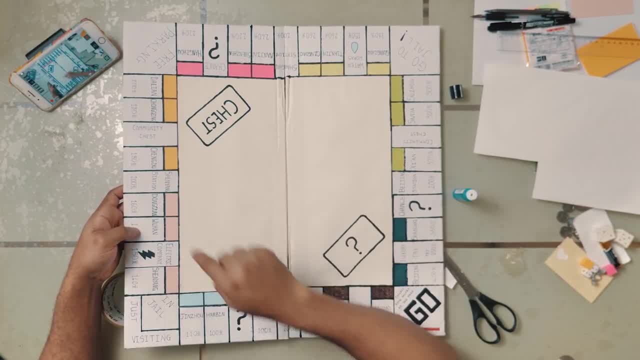 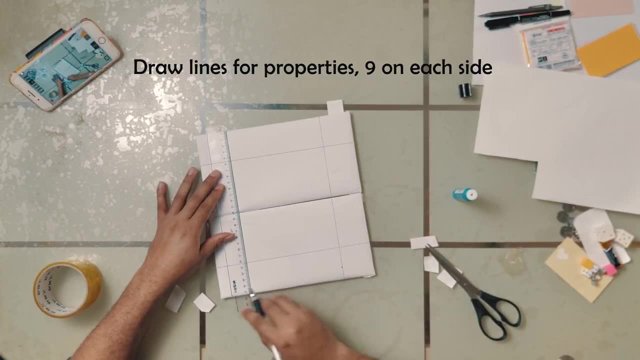 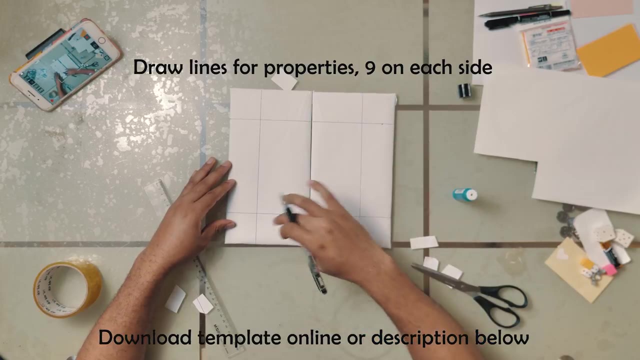 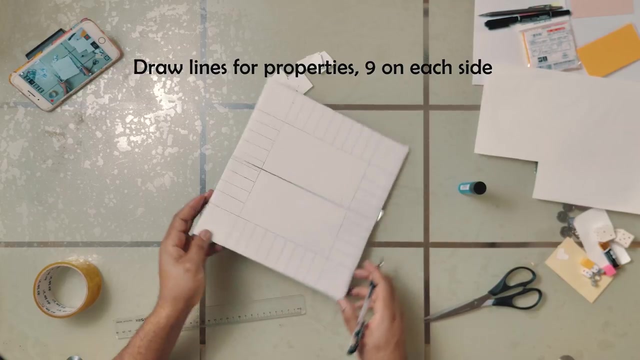 As you can see what we have here. So we're going to draw each of the properties with our rollers. So each of this piece, the properties you have like nine, nine properties in between. The next thing I want to do is add in the colors. 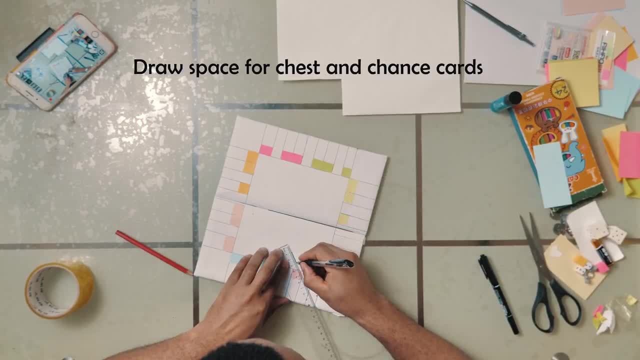 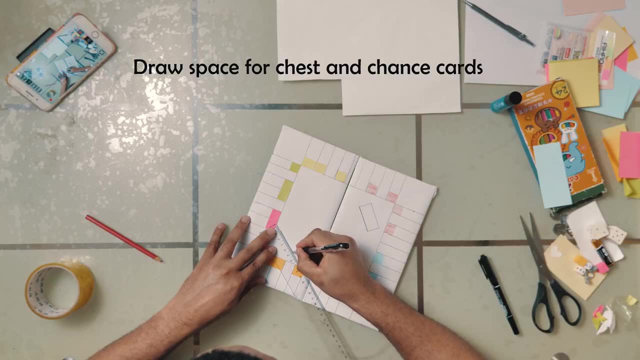 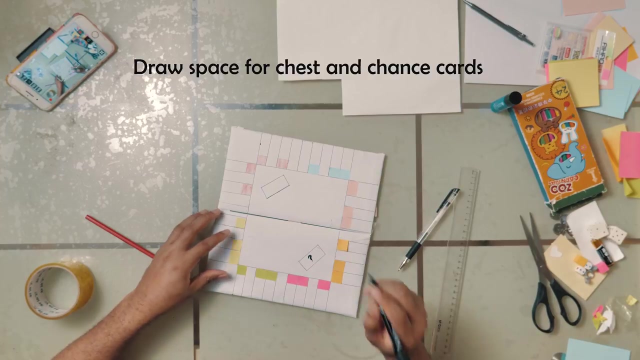 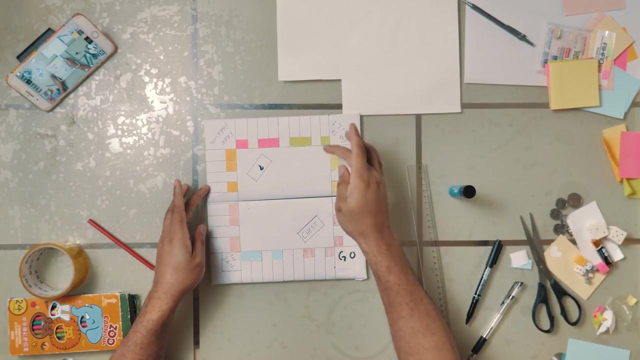 this is how I made my board. as you can see, I made sure the different properties are of different colors, while you have to go go to jail- free parking and go to jail, which is gonna bring you down here. so this is the final look of what it. 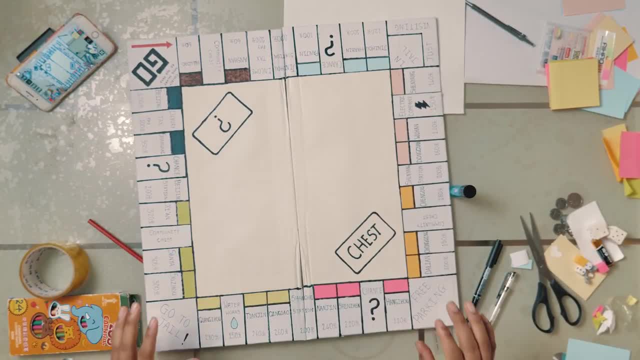 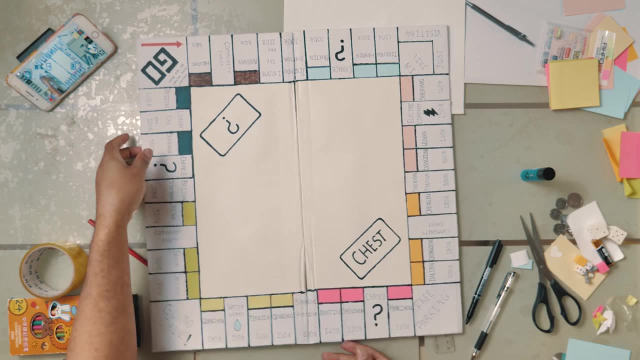 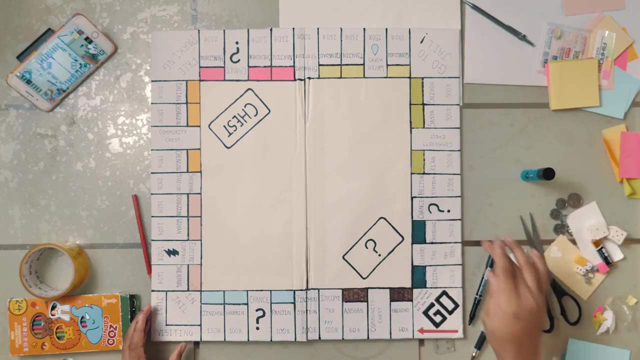 looks like haven't named the cities according to the cities which are more familiar with. since I'm in China. I'd say to label my cities according to the cities in China, from my most expensive houses or properties, which is in Beijing and Shanghai, all the way down to the least house, which is in Uludao and Anshan. 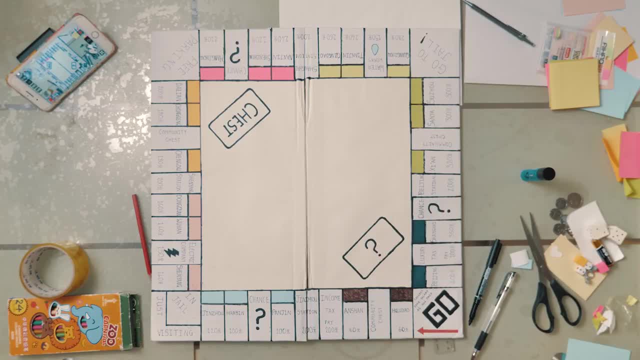 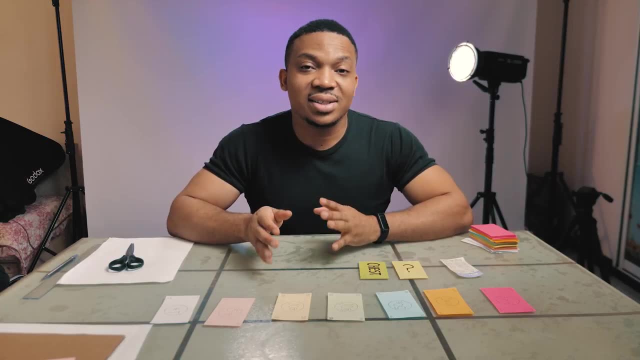 so this is how you make your board. you can do it whatever you have at home, easy and no stress in making the money: property cards, community chairs or channels. this is a section where you're gonna be doing a lot of cutting and a lot of writing too, so I've chosen different colors of papers to make my own money, because it's 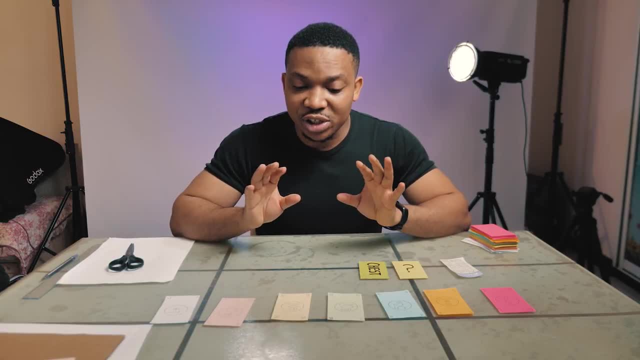 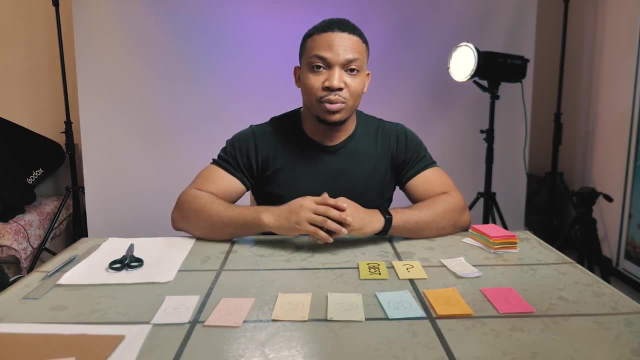 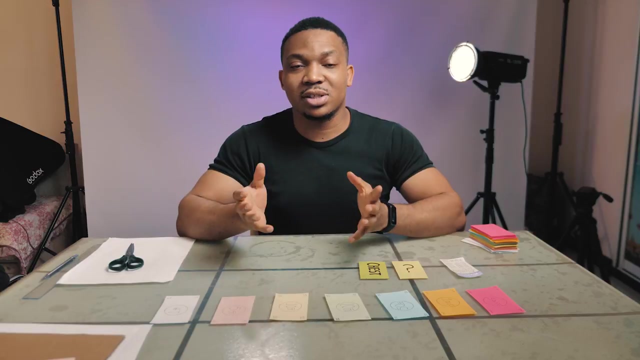 very important for you to be able to differentiate these colors immediately when you see them. it's easy when the banker is giving out the money and you can tell when playing with other players too. I chose RMB because I'm in China. you can choose any currency you want: could be US dollars, naira, kwacha and whatever. 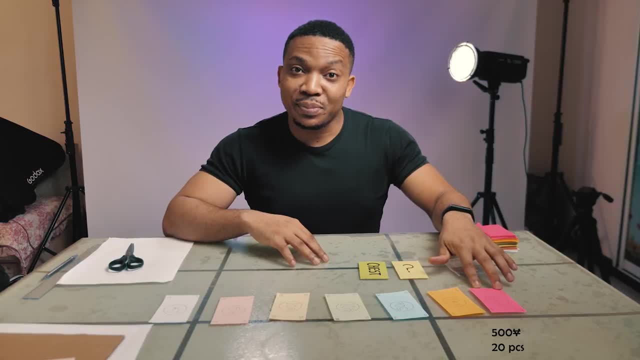 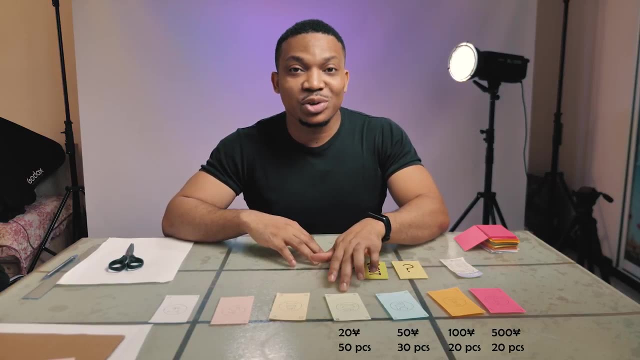 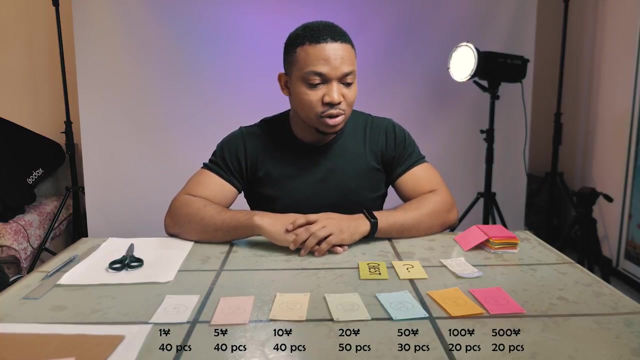 country you're familiar to. for five hundred, you need twenty pieces. four hundred, you also need twenty pieces. for fifties, you need thirty pieces. for twenties, you need fifty pieces. for ten, five and one, you need forty pieces each. so just go ahead, get your paper, cut them. 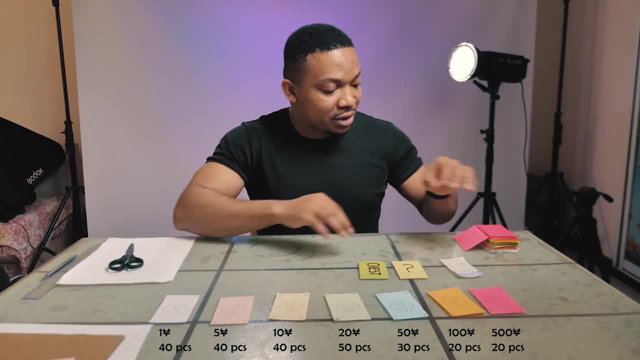 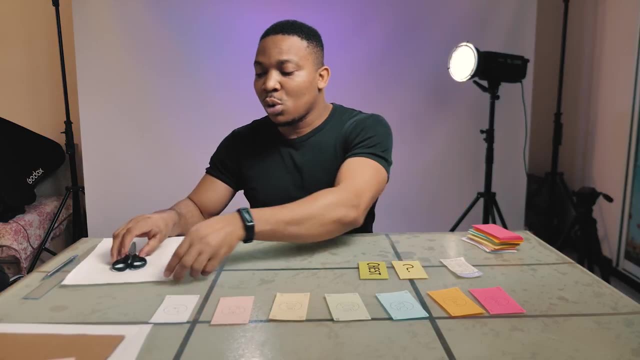 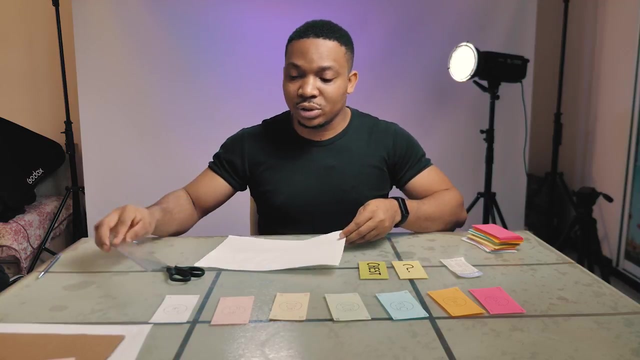 make sure the dimension of each of this paper are similar, because it's easy for you to stack them, like I have here to stack them, and you're good to go. so I'm just gonna use one example here. here I'm showing you how I cut them. I already used my ruler to measure out this dimension. 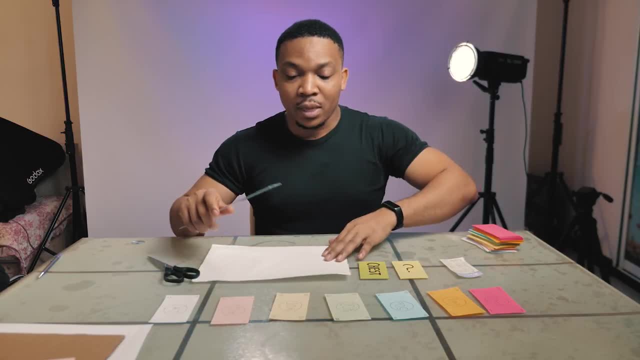 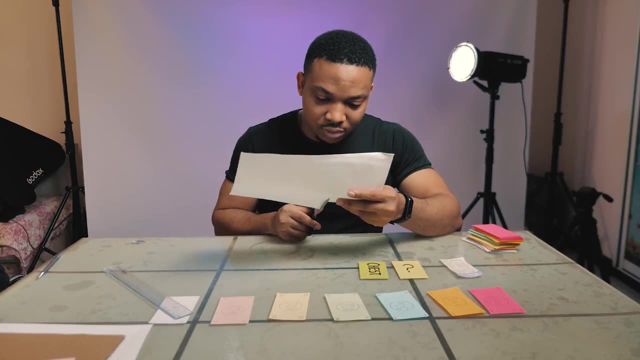 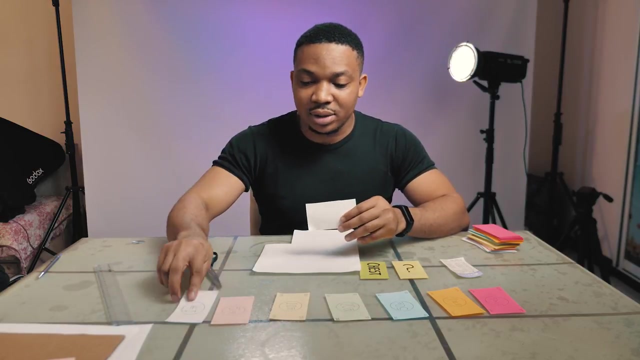 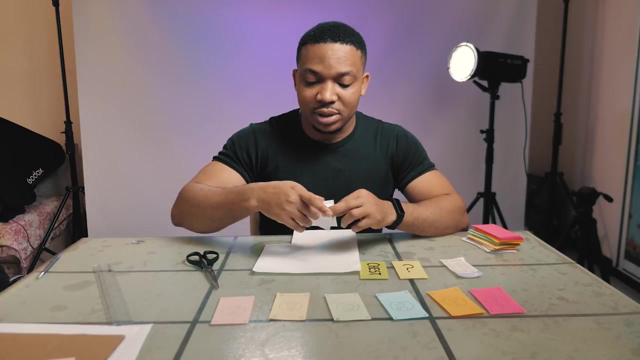 so it remains consistent in all the money. So you measure them and you cut them equally. So, yeah, that is how I made. I cut them for the ones and all of them. So you can just do that, go ahead. and I made a circle in the center, as you can see here, and I wrote the. 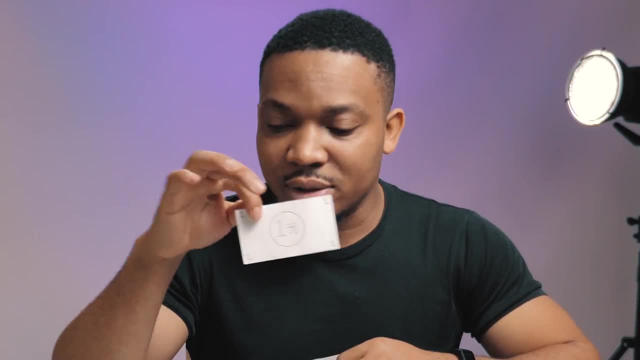 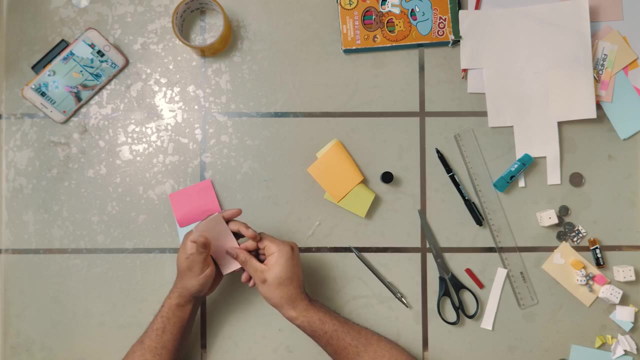 currency and also what is the value of it. So go ahead and do that for all of them. For the community chance and chance card, you can use the same piece of paper which you use in making your money and also designing your board, But I made a little adjustment. 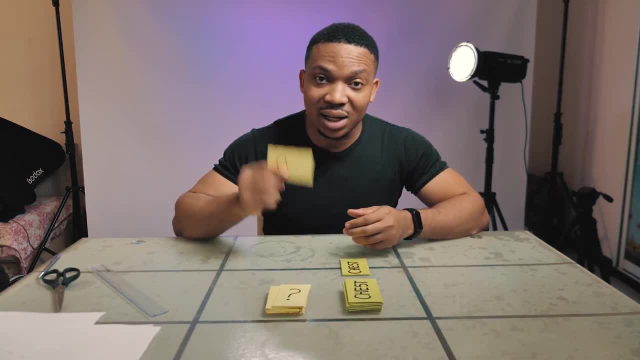 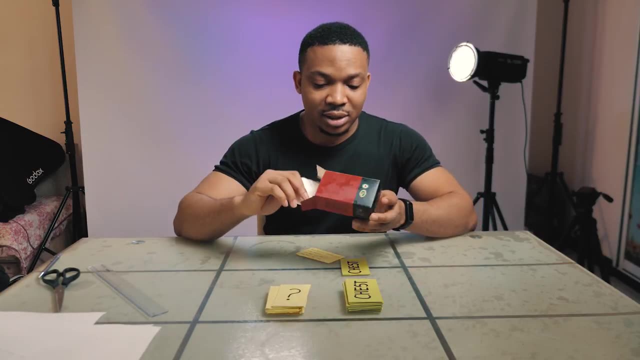 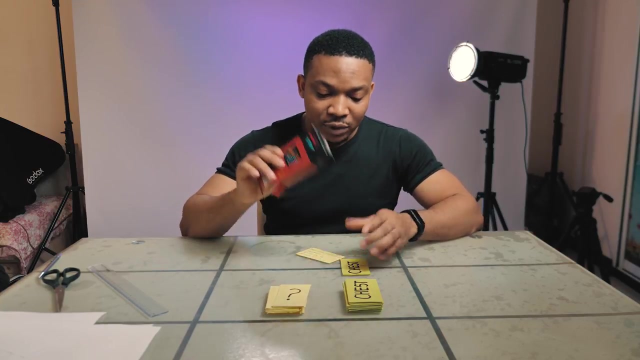 because I felt the texture or thickness of the money and that of the cards should feel a little bit different. So I got from my tea the box of one of the Chinese tea. You could use that of toothpaste, you could use that of spices. whatever you have cut them, exactly the same shape Place. 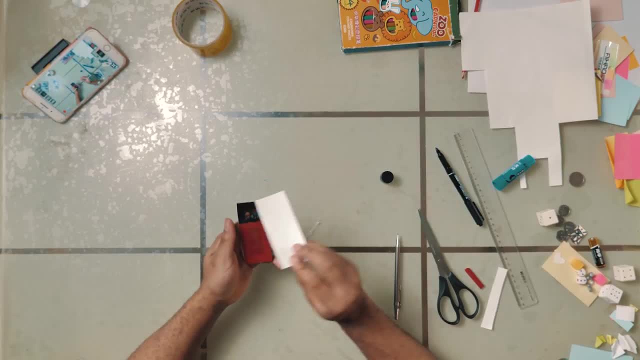 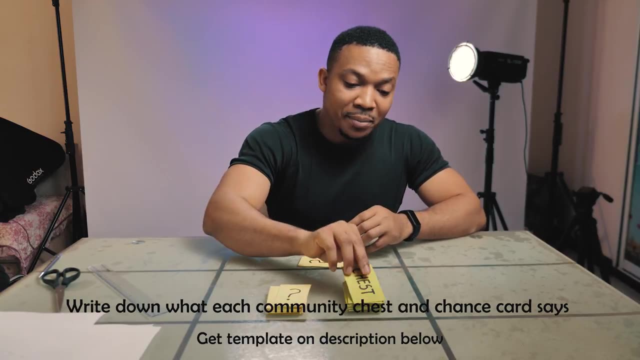 two of your papers in between and you glue them. and here we go, Your community chest and your chance card, and they feel very strong and rugged. and it even makes it more fun because when you pick it up from the card you see it's more firm. 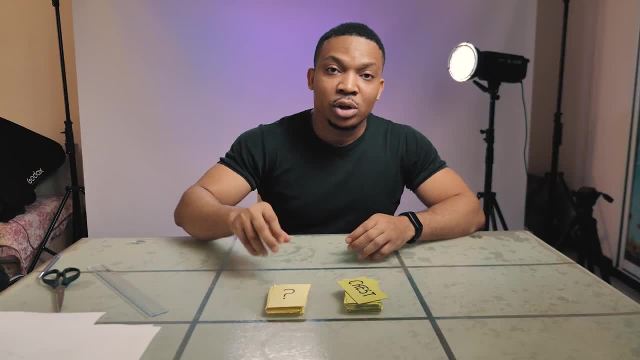 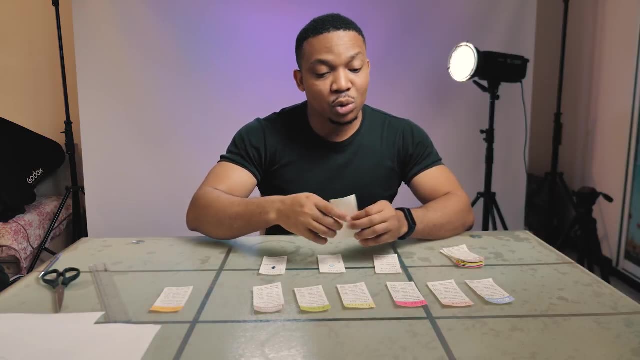 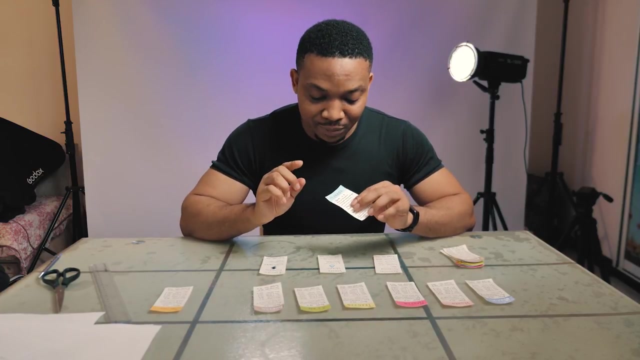 and it's easy for you to reach. So, moving forward to the property cards: For the property cards, you also need plain piece of paper and also you will need to cut these papers in equal size or dimension and note or have in back of your mind that you need to color each of these papers in different. 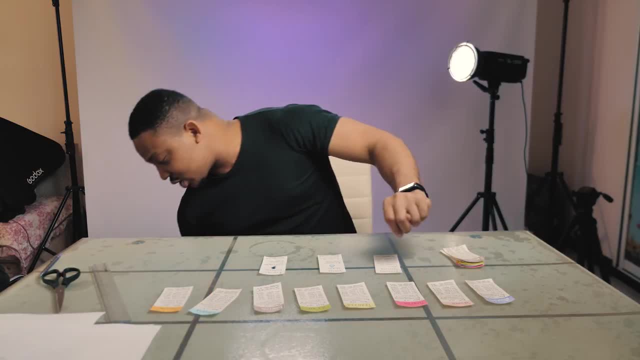 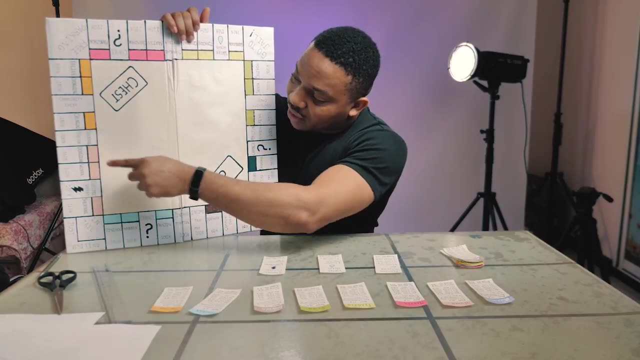 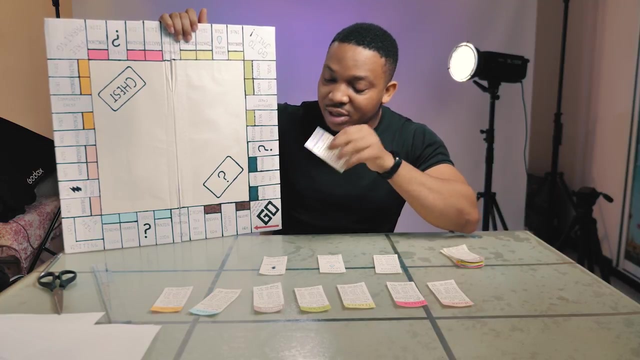 colors that matches the colors of the properties which they represent. So, as you can see, my board, Each property has different colors. So let's say, for example, and my most expensive house, which is in Beijing, Shanghai, I colored them with blue, even if it's not a perfect match. 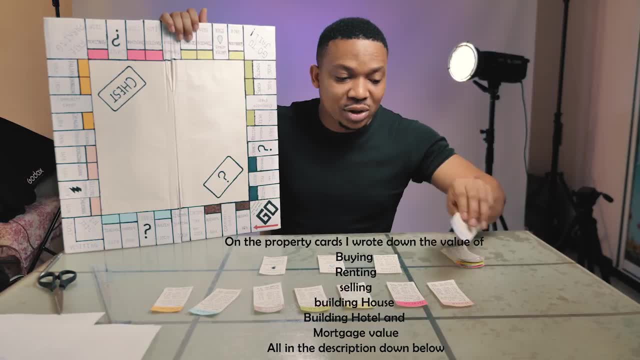 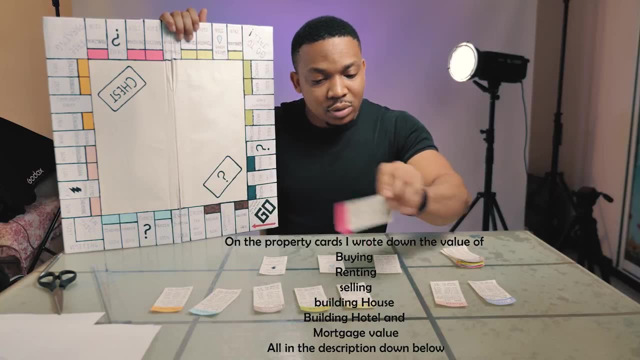 but this is the closest based on the materials I have. So I keep stressing: you can get creative and use whatever you find around you. So you color this according to the um. the color of the property should match that of the card. 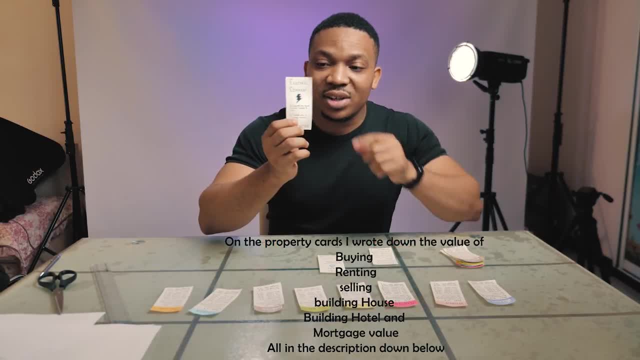 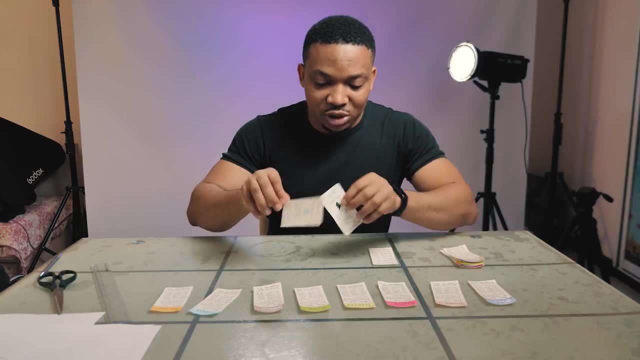 Don't also forget that of the card. Okay, The electric company. you can see my little um light stone which I've made here just to make it different, And also my water workstation. And last I have the train station. 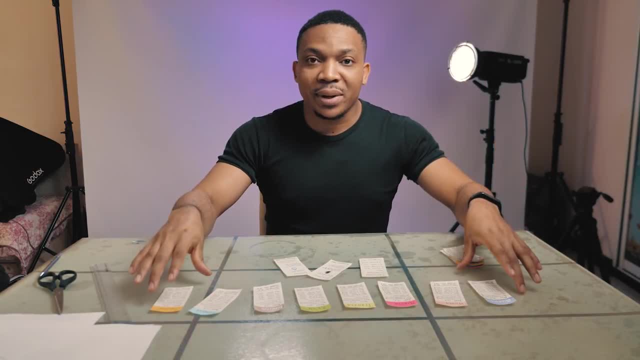 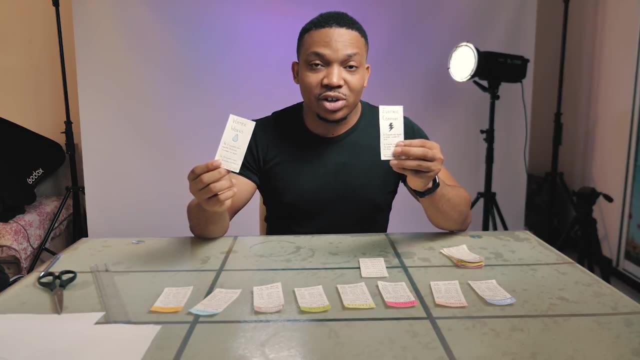 So you will need each of this um properties- about 26 of them- And also for your utility, which is your quarter and your um electric company. you need two of them, And also you need four train stations. So that's it with the um. 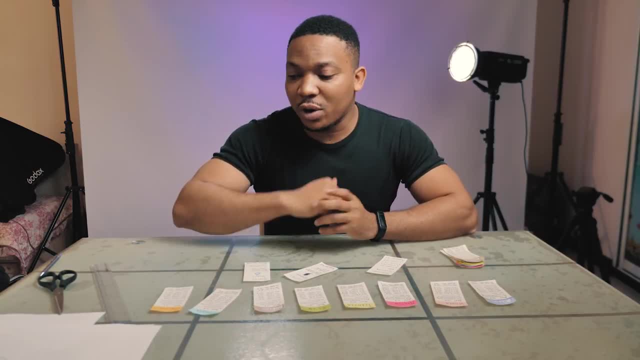 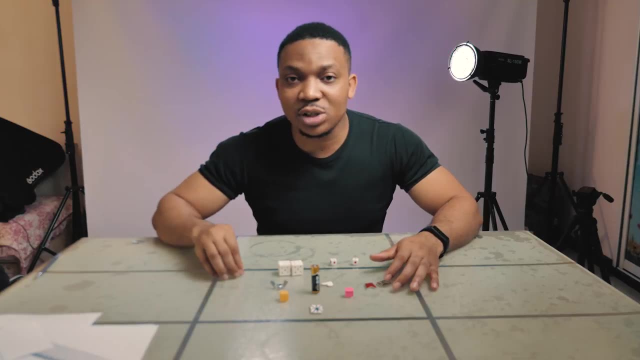 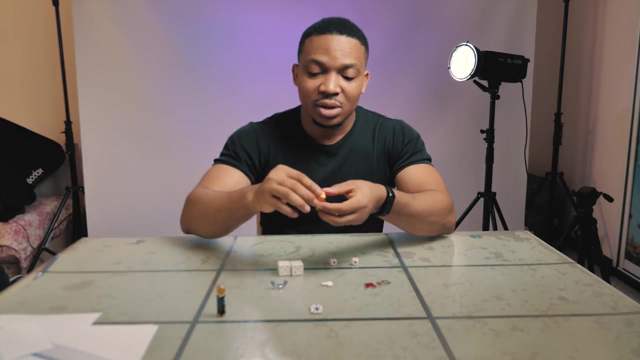 property card and utility cards, moving forward dies and token. So basically the token is anything you can use to move from one point of the board to another point. So I have your batteries you could use to move, or these are erasers which I caught. 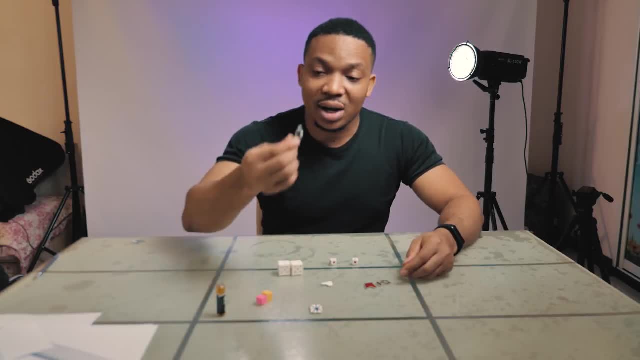 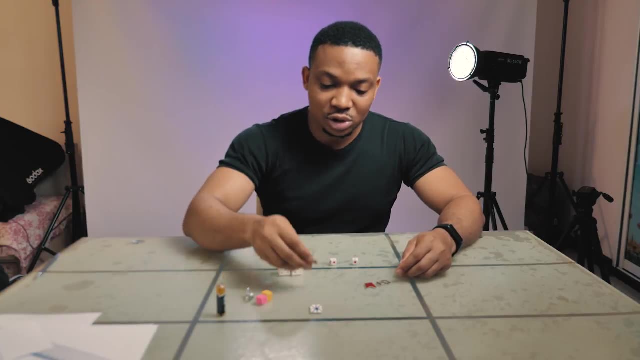 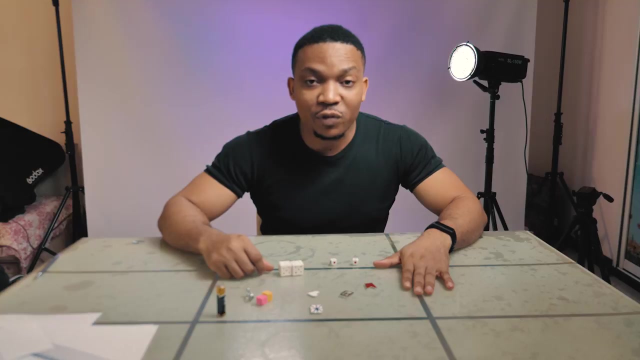 um, and covered up with colored paper. I also have this, which just a screw could use to move, and you have a piece of paper which I caught into the shape, Um, the heart, anything you could use, So any piece you find around your house to move from one point to another. 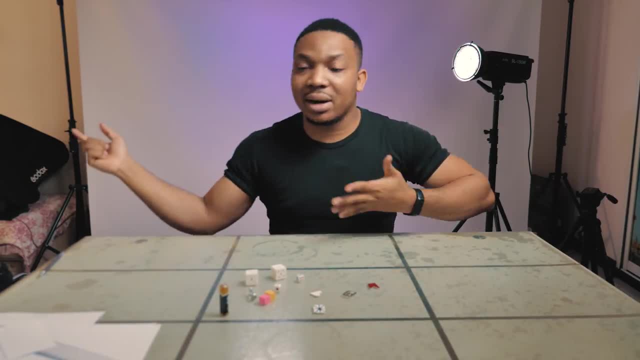 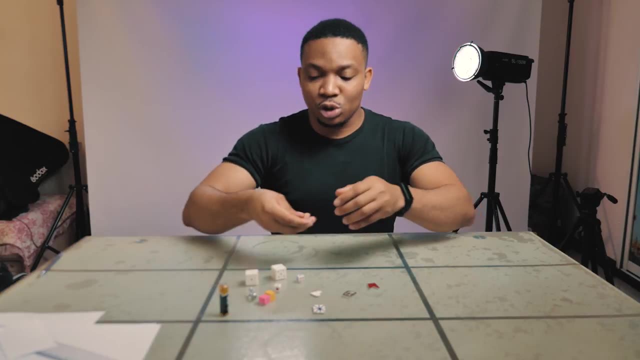 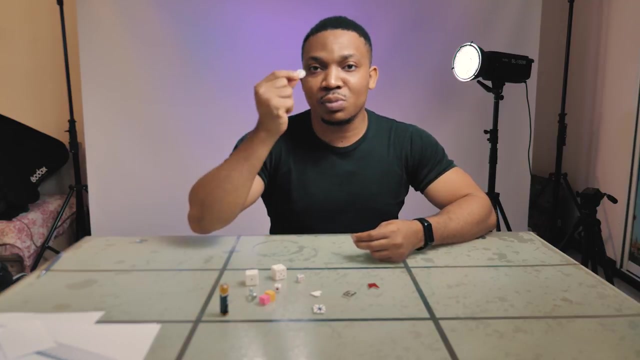 So for the house and hotels you will also need anything around you to differentiate when a player buys a house and when a player buys a hotel. So I've said to use different sizes of coins to indicate my house and hotel. So I've used the smaller coins for the house, because I need four of them. 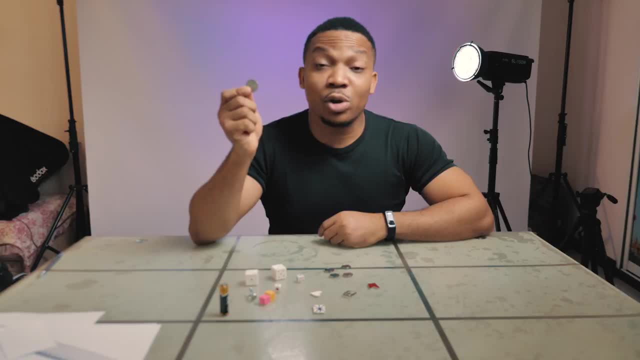 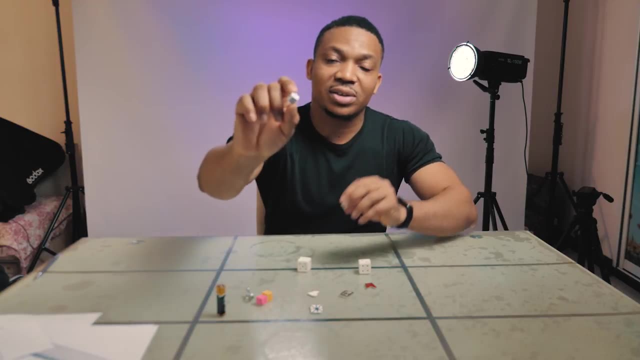 And I also use the bigger coin for the hotel. concerning the dice, If you don't have these, um original dice, or which came, which comes with the monopoly, or any other form of game which you play which you need to roll a dice. 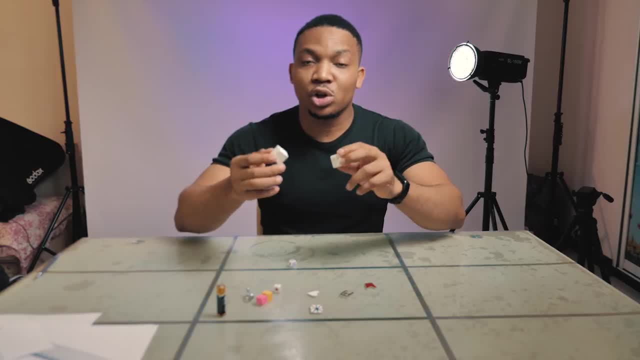 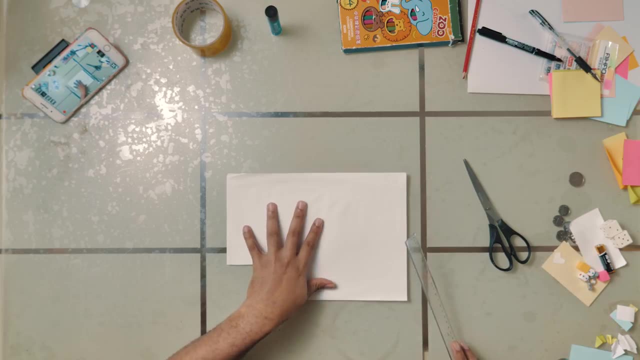 You can also make your own dice. It's very simple. I'm going to show you how I use a plain piece of paper to make my own dice. So you're making the dice. You will need a plain sheet of paper, Okay. 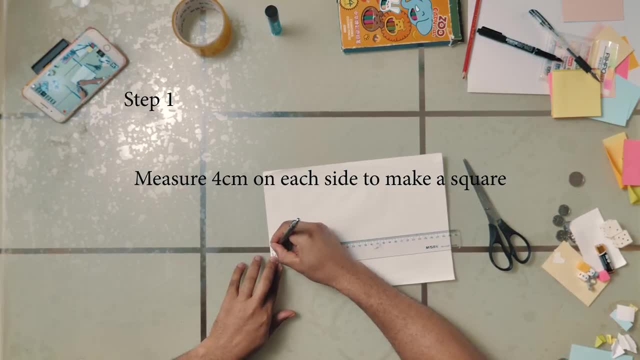 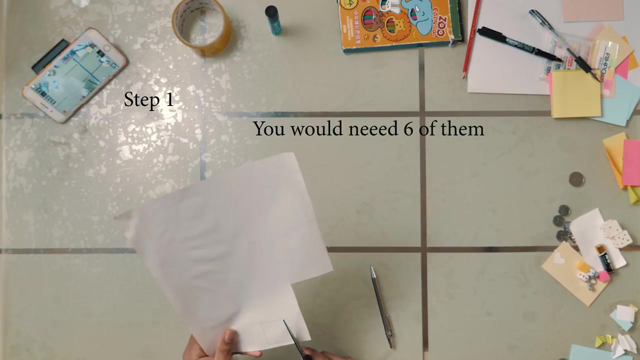 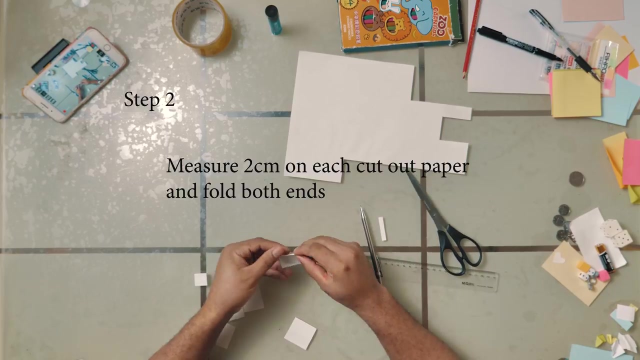 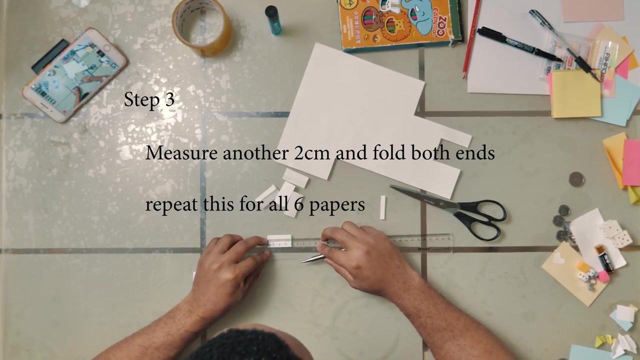 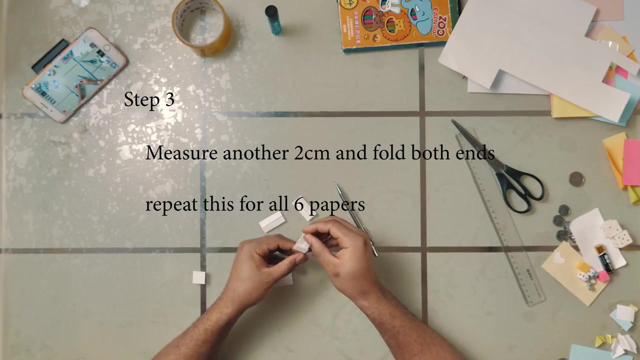 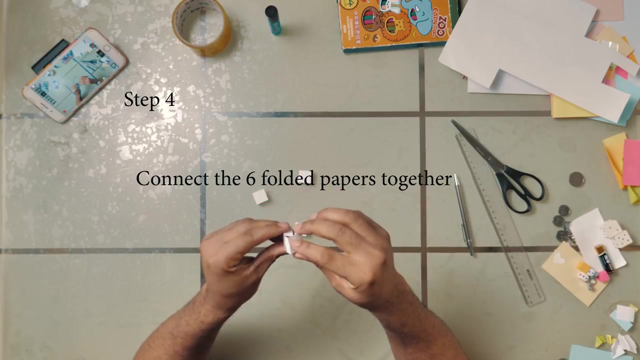 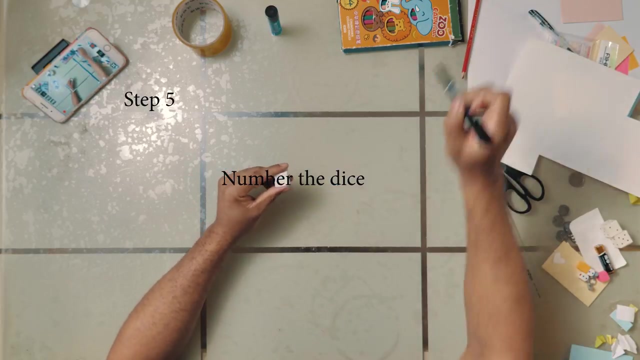 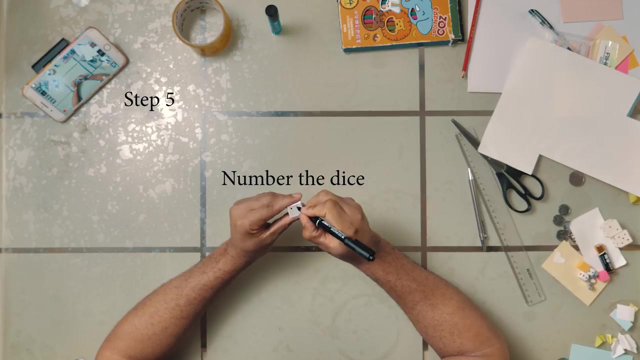 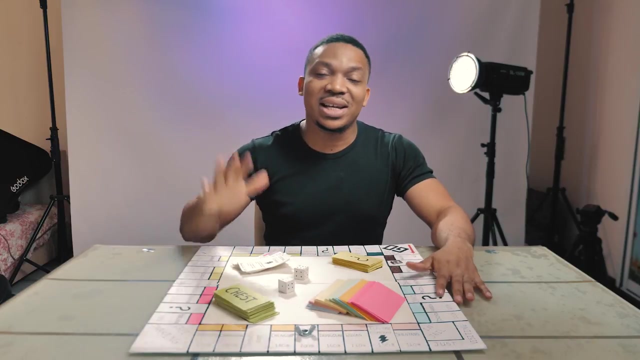 And you have to measure four centimeter on one side and also four centimeters on the other side. Thank you, Thank you, And that is it, guys, your simple DIY Monopoly game. This was very fun making and I'm sure you guys are going to have a lot of fun making it too. 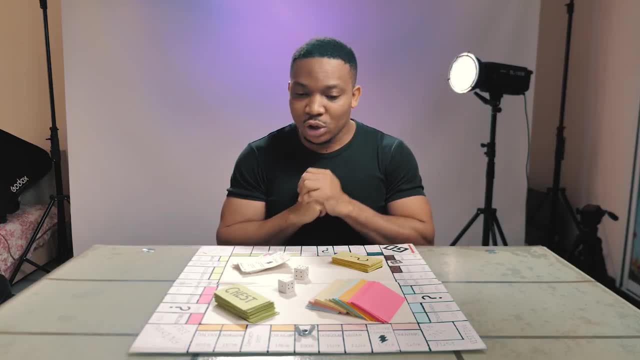 Using simple materials, tools you find lying around your house, And this will come very handy, especially in this isolation period. Something to do with the kids, something to do with your partners, your friends and your loved ones. So, if you have any problems or if you have any issues, making your own game. 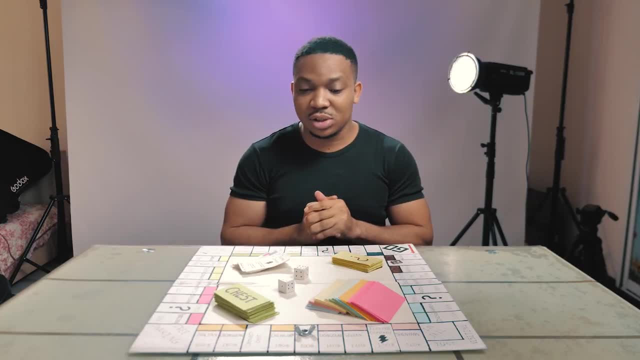 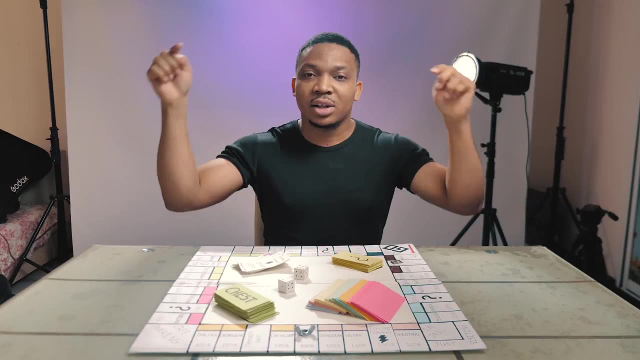 please leave a comment in this comment section down below and tell me the difficulties you had making yours, And if you have better suggestions on how to go about making this, please feel free to leave it also in the comment section down below If you are new to this community. 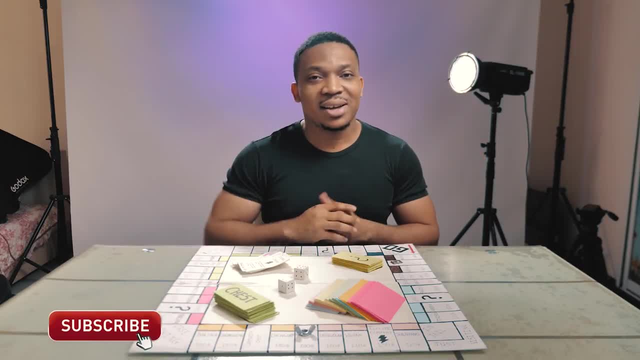 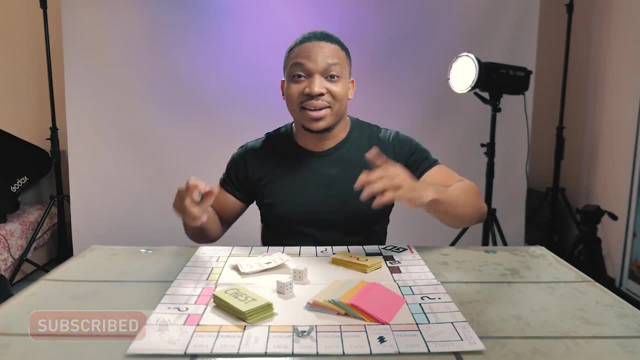 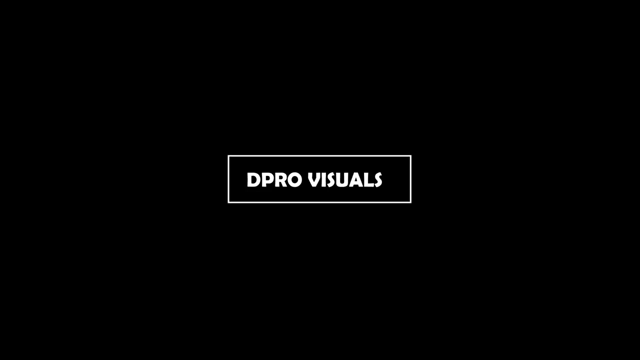 and you've not subscribed to my channel. please don't forget to subscribe and click the notification button so you get notified whenever I upload new videos. And remember it's either you go pro or you go home. Bye for now. Subtitles by the Amaraorg community.